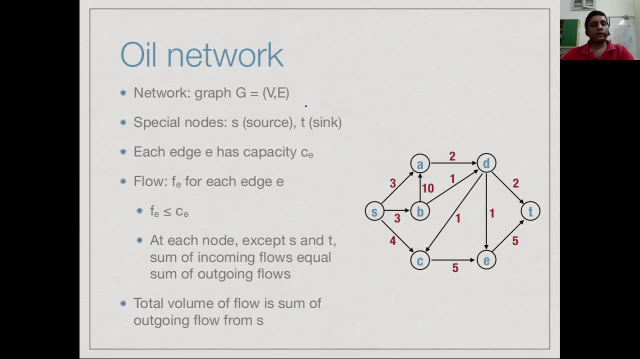 So the problem- just to phase it, phrase it formally- is that we are given a special demand, So we are given a special demand, So we are given a special type of graph. So it is a directed graph and it has two special nodes: a source and 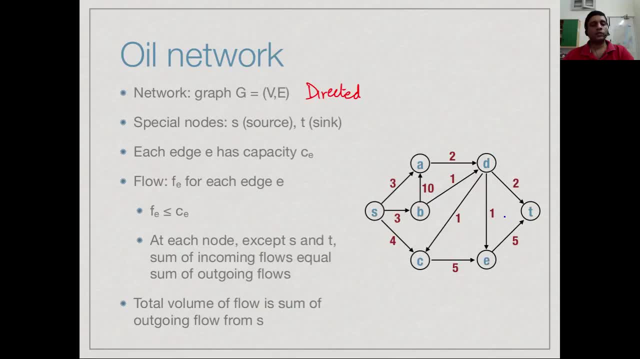 a sink. The source has no incoming edges and the sink has no outgoing edges. Each edge has a capacity, which is a weight associated with it, and our aim is to come up with the flow. A flow is again a quantity that we will assign each edge. and now the flow must satisfy. 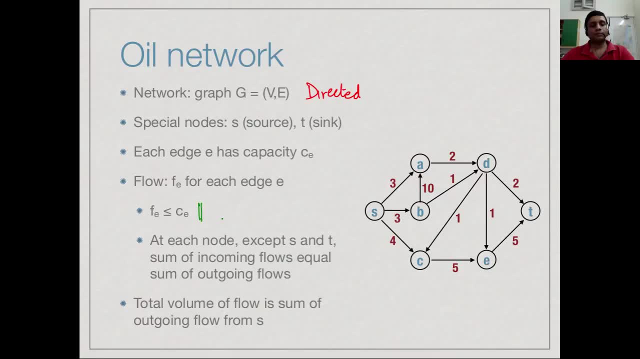 some basic conditions. The flow must always be less than the capacity. Then we have no storage. So at every internal node the total amount flowing into the node must be equal to the total amount flowing out. So this is called conservation of flow. 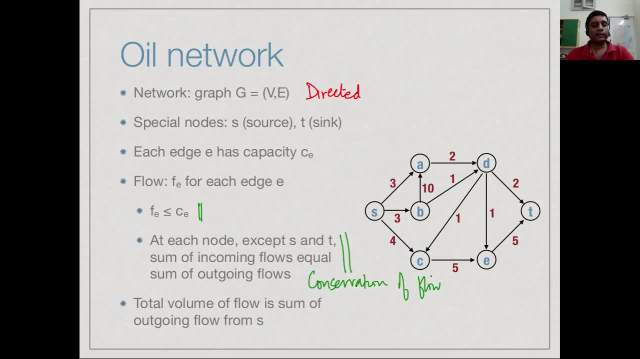 We cannot lose anything or generate anything at an intermediate node. everything that comes in must go out. And, finally, what we want to do is we want to optimize the total volume of flow, and the total volume of flow is the amount of flow which is coming out of here, which is also, of course, the amount of flow which 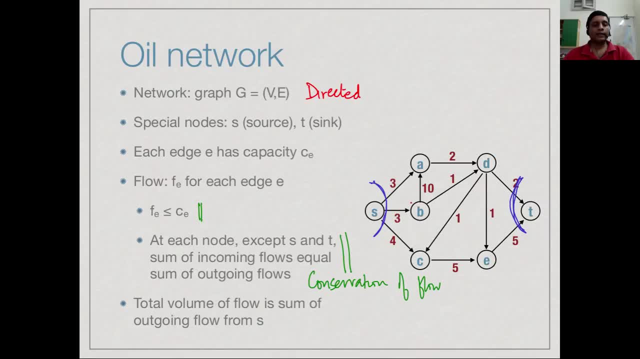 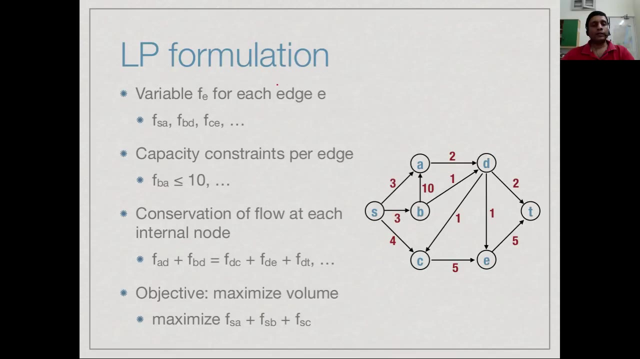 is going there because no flow can be lost. ok, So we can look at either end, but let us just define it to be the total volume of the outgoing flow from the source node. ok, So now we have this formulation in mind, So we can now set up a linear program for. 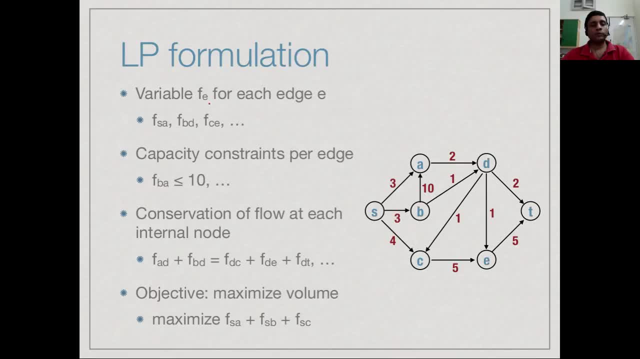 it right. What we associate do is we associate, as we said, one variable for each edge. So, for instance, for the edge for SA, we have FSA, and then for the edge BD, for example, we have FBD, and then for CE we have FCE, and so on, right? So we have 1,, 2,, 3,, 4,, 5,, 6,, 7,, 8,. 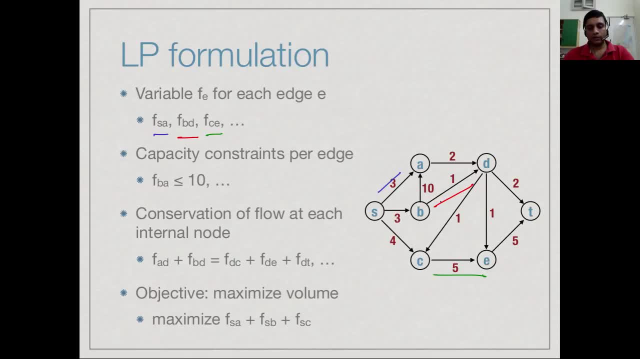 9,, 10,, 11, I believe, edges, yeah, 11 edges, and therefore we have 11 variables in this linear program. ok, Now, what can we do with these variables? One first is: we can say that each variable is constrained by a linear program. So we 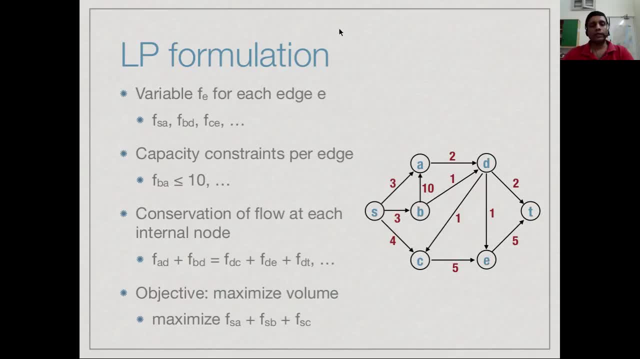 have a capacity of the corresponding edge. ok, So FBA. So BA is now this edge. it has a capacity of 10.. So whatever flow I finally arrive at from B to A must be less than 10.. The other thing that we can say is that we must have a conservation of flow at each internal. 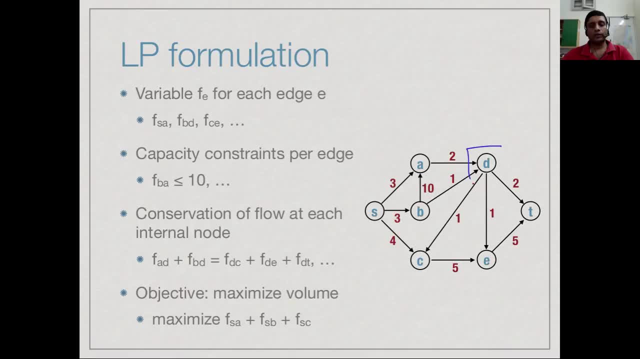 node right. So, for instance, if I look at this node D, then the incoming flow is AD plus BD and the outgoing flow is DC plus DE plus AD And these 2 quantities must be equal. FAD plus FBD must be equal to FDC plus FDE plus FDD. 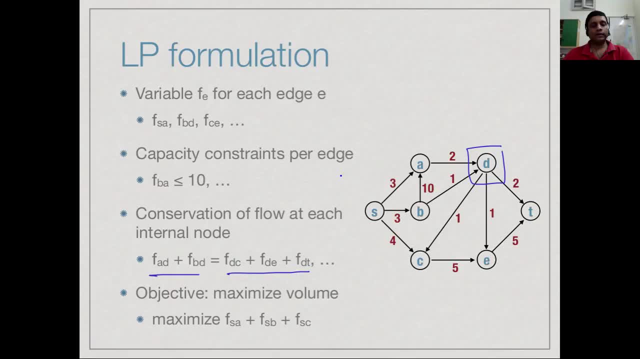 and finally, So these are the constraints, right, The constraints say that every edge can only carry a flow within its capacity and every internal node, there is conservation of flow And, finally, our objective is to maximize what happens on these 3 edges. FSA. 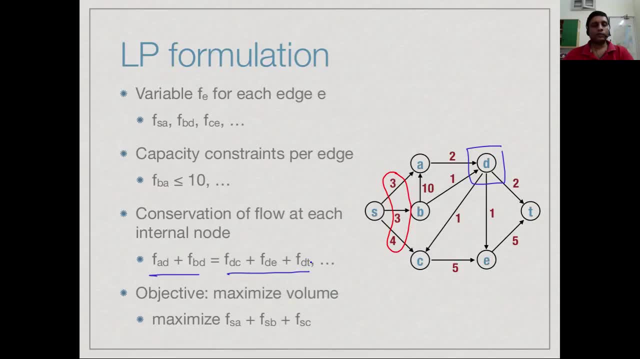 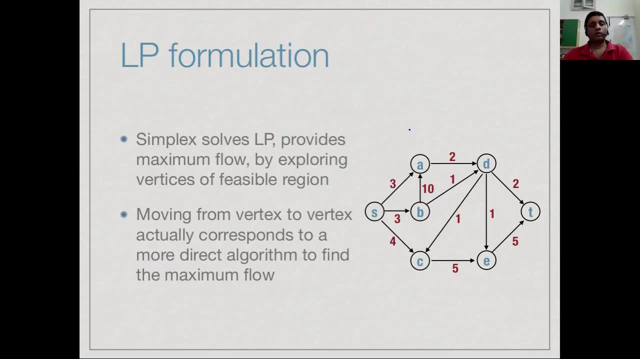 plus FSB, plus FSC. ok, This is our objective function. So, of course, as before, we will just invoke a linear programming solver such as simplex on this and get an answer. But what we will do now is to understand what this actually means, Remember how simplex works. So simplex starts at a vertex in our 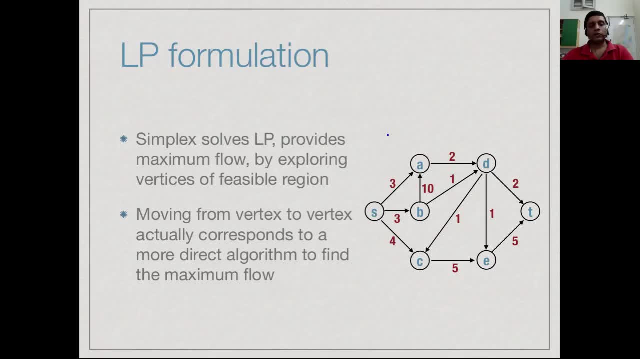 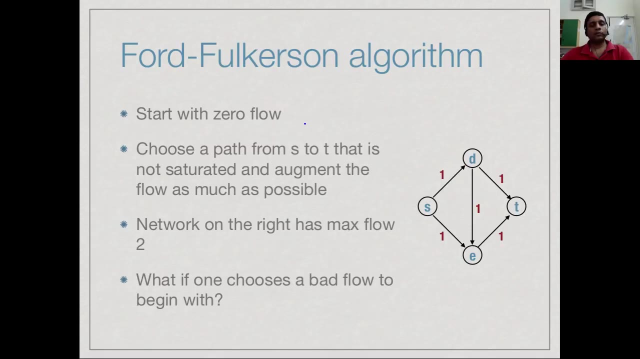 feasible region keeps going from one vertex to the next. So as long as it is increasing the flow, ok. it is actually taking an existing flow and adding something to it, And this can actually be interpreted directly in terms of a flow finding algorithm. So there is an algorithm called the Ford-Fulkerson algorithm, which 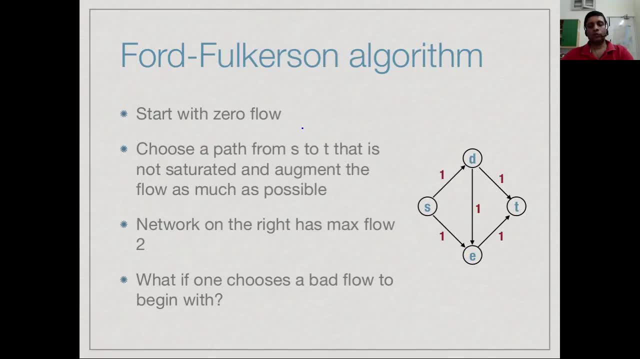 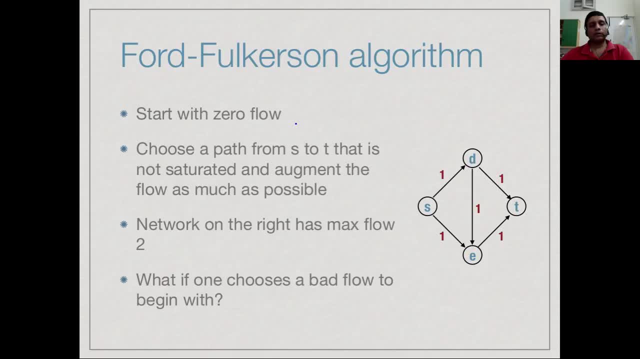 what we are going to do. So now, if you you look at the network on the right, it is very clear that there is a flow possible here. you can send 1 unit of flow that way. you can send 1 unit of flow this way. Therefore, the full 어�kerson algorithm says: take any path which exists and start flowing things to there. So you could, for instance, to begin with this path, the one that goes to S to D, and then from D down to E and then to D. So this programming is going to be done in this way. And then all these blocks of y point which we have, training less 살짝, we can Continue to take lessons. 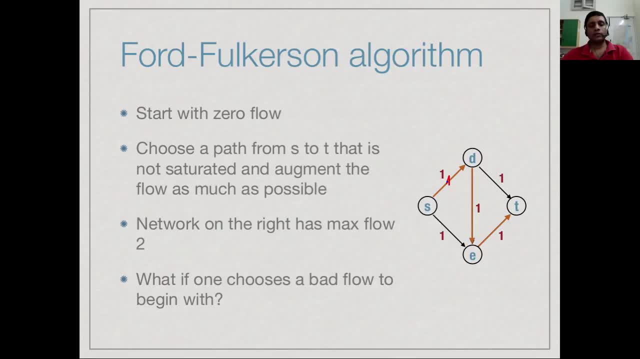 flow is one unit, but now, at this point, this edge is now saturated and this edge is now saturated and of course, this edge is in the wrong direction, So I cannot make use of these two capacities to generate the second unit of flow. So it looks like the Ford Fulkerson. 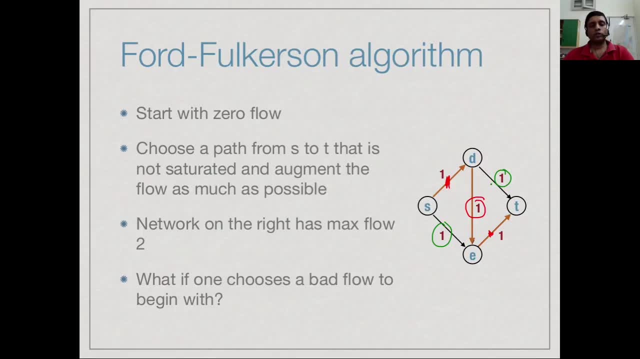 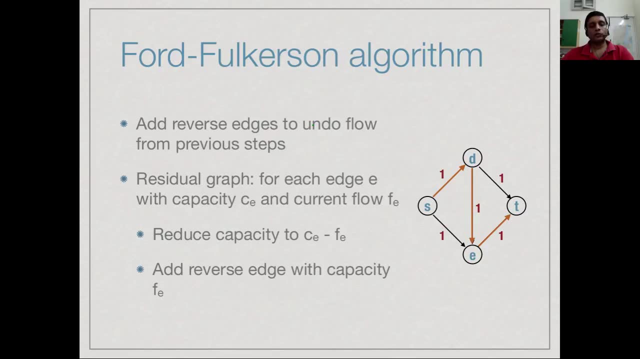 algorithm reaches a bottleneck if you choose the wrong path to start with. So the solution is to say that, even if we have taken a bad path, one of the things we can do is reverse the decision we made earlier. So we want to say that if we are flowing, 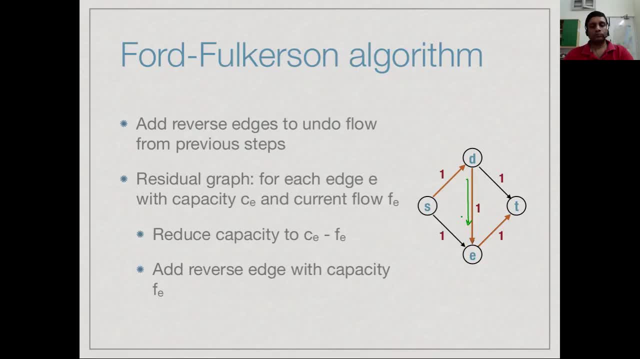 one through this, then we can reduce this flow, So we can divert this flow back another way. So that is a bit complicated to describe, but one way to solve it is to actually set up an extra edge allowing us to flow things back. 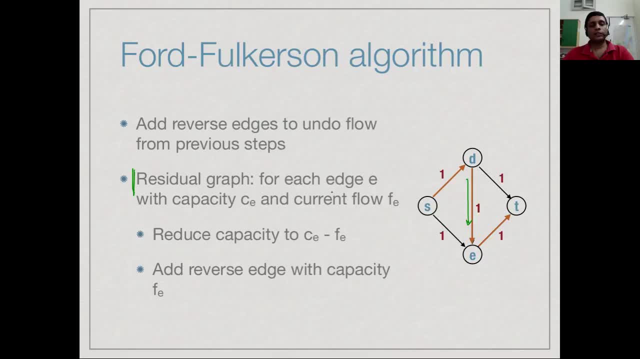 So this is the solution. So the solution is to say that, even if we have taken a bad path, one of the things we can do is reverse the decision we made earlier. So this is what we call the residual graph. So in the residual graph, what we will do is we will 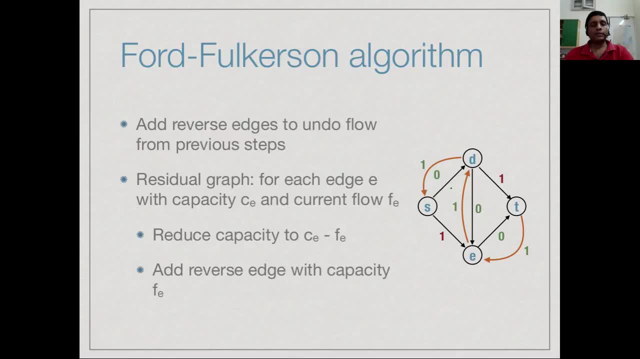 actually take the flow that we just constructed and then we will change the capacities. So the forward edge S to D, which had capacity 1 and flow 1, now has residual capacity 0. So if we have a regular edge, then we replace its weight by the actual amount that is still. 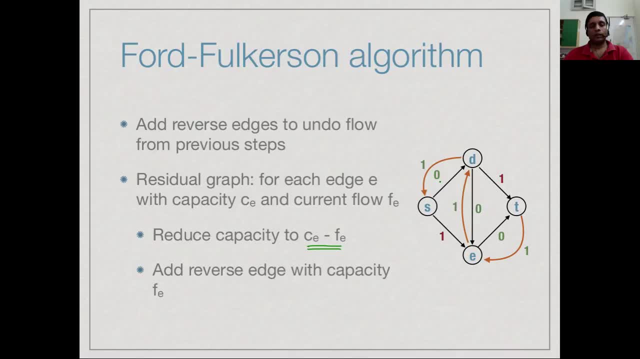 available. So that is the capacity minus the current flow, And in addition we add these new edges, these backward edges, which correspond to the flows that we have committed but which we may want to change later on. So we have sent. 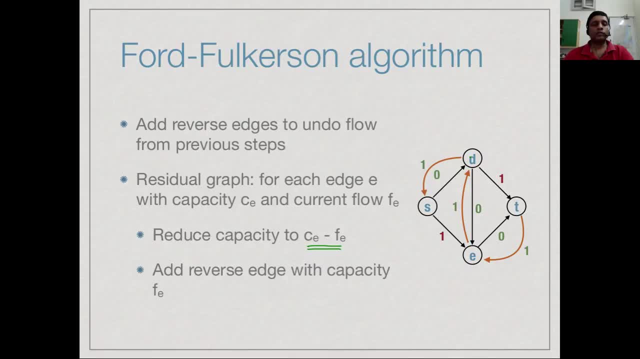 a flow 1 from S to D, but now we can reduce that flow by sending some flow back from D to S. So that is what it is supposed to be So formally. this is how you construct the residual graph: You take the original graph, then any flow that you have set up in an existing 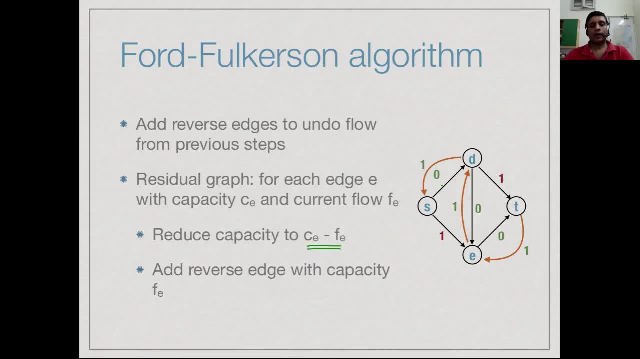 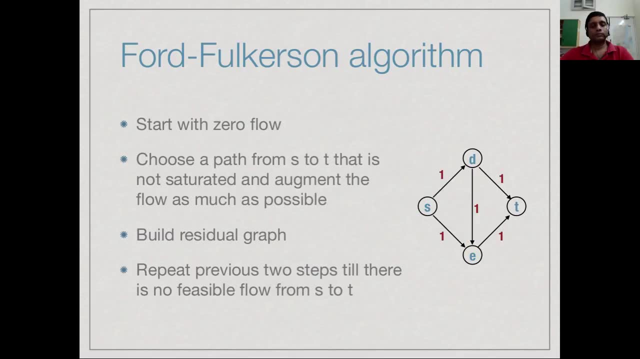 edge, you reduce the capacity of that edge by that flow And, corresponding to that flow, you set up a reverse edge which allows us later to undo this. So, going back to this example, so what we would do is we would first start with this. 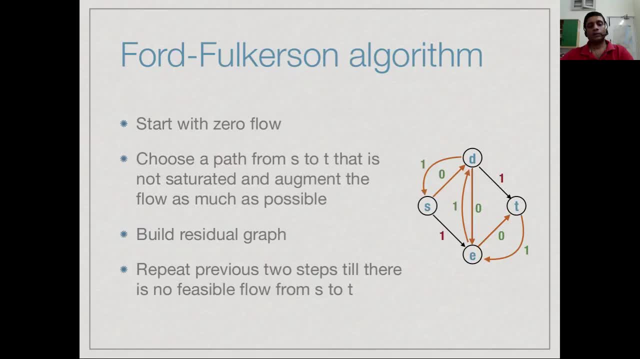 wrong flow, And then we will say R, but then we will build this residual graph And now we will observe that in this residual graph there is a path which goes like this. So we are not talking about the original graph, we are only talking about the residual graph. 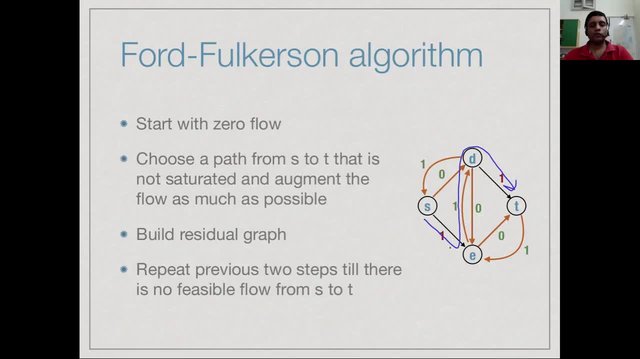 at each stage, So we would build this Now. this will result in a new flow, So this will end up producing a 0 here, a new edge back here. similarly, a 0 here, a new edge back here, And this 1. 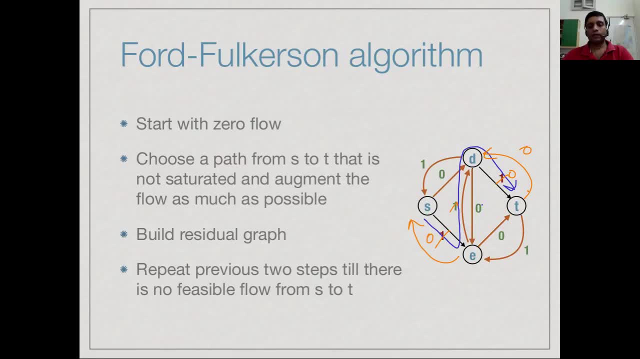 will now become cancelled out, because now this path is this flow, so this is restored to 1 and this edge will disappear. And now in this new graph, we will find that there are no edges left, because I have 0 capacity going from S to D. I have 0 capacity going. 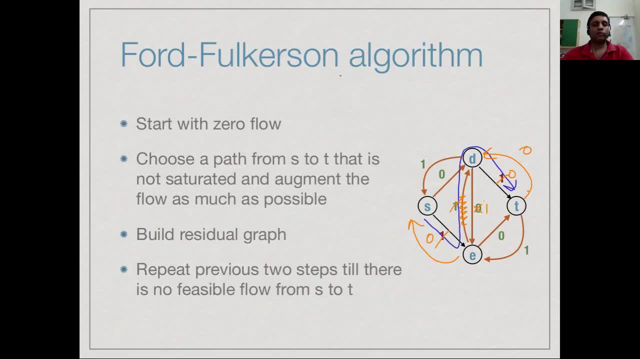 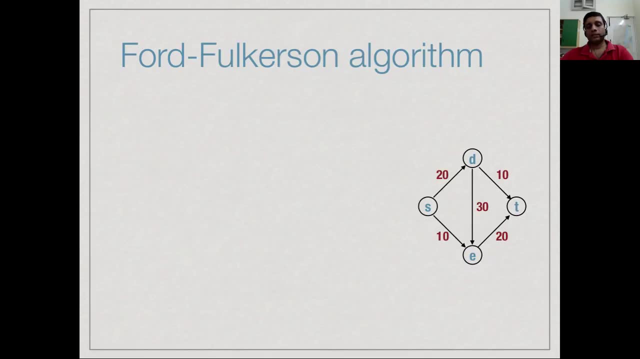 from S to E. I cannot leave any flow of mass, So this is my final field. So this is the Ford Fulkerson algorithm. Let us look at it again in a slightly similar structure but with a slightly different set of numbers. So this is a graph which has not 1s, but some 20s and 30s. So here, 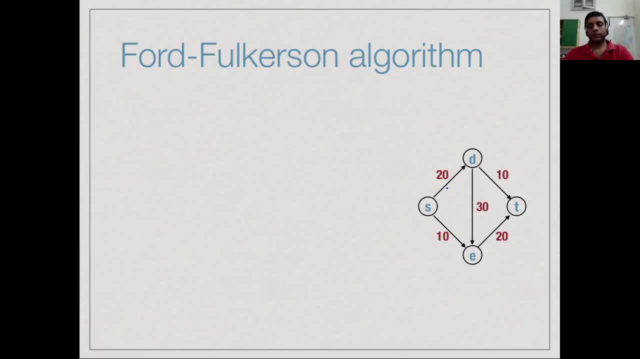 intuitively. the claim is that all 30 units can flow, But the 30 units cannot flow- unlike the earlier case- along the edges of the diamond, Because if I take 20 units up then I must split it as 10 plus 10.. So I must recognize that 10 must go down and 10 must go there. 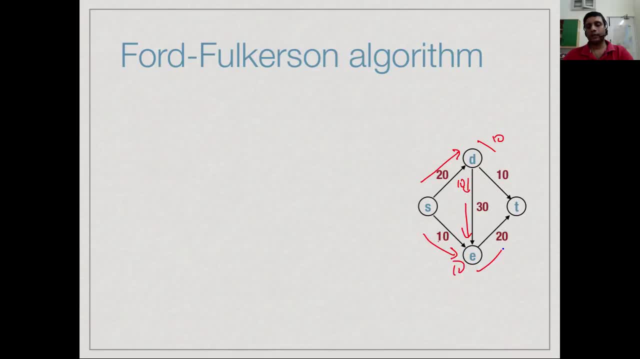 Similarly, if I put 10 here, then this 10 and the incoming 10 combine to form this 20.. So this is how I get a flow of 30 in this graph. But if I start the Ford Fulkerson algorithm, 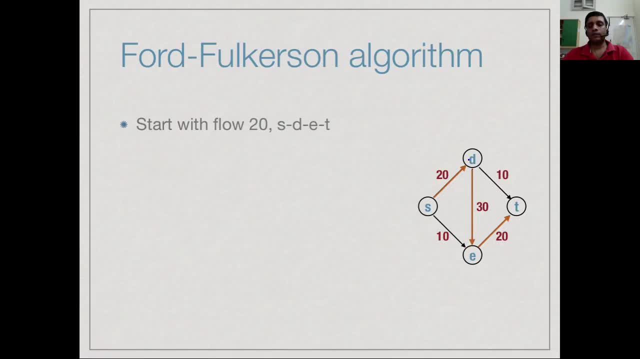 it will try to saturate a path. So, supposing it identifies the path s to d, to e, to t, Then if it identifies this path, then it has put a 20 flow through this edge. So we start by this flow and we build the residual graph. Residual graph says that this: 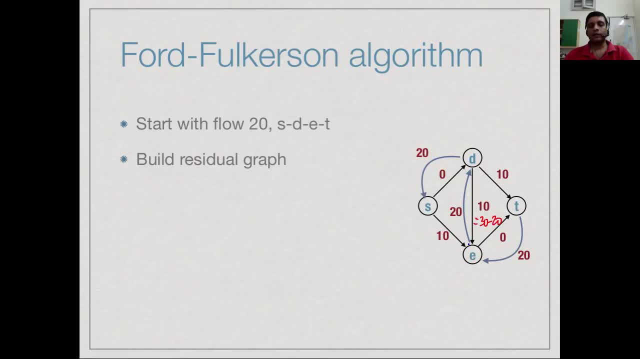 10 is 30 minus 20.. The residual capacity from d to e is now 10, because I had a capacity of 30 and I have put 20 through And the blue edge is now the residual edge, which allows me to reduce this 20 back. Similarly, from s to d, I had earlier capacity of 20.. I have 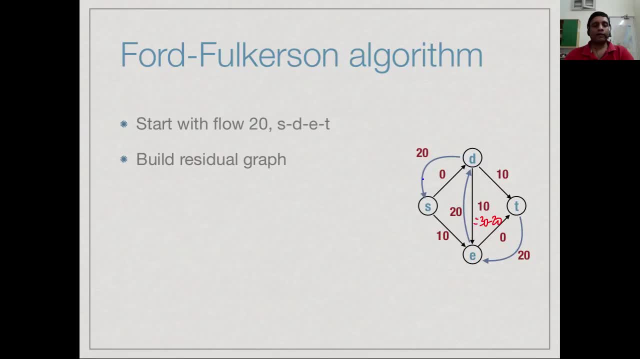 put 20 through it, So its reduced capacity is now 0.. But I have a backward edge which I am going to undo this later if I want. And the same with e to t. e to t has reduced to 0, but I have a backward edge. Now I look for another path in this graph. 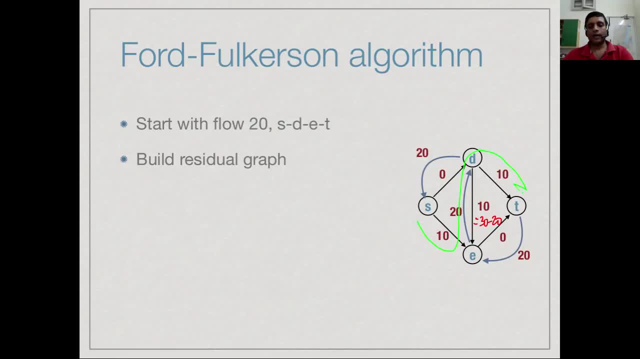 So, for instance, I find that this path is there. I have a path from s to e to d to t And s to e to d to t. my constraint is 10, because I have only 10 flowing out of s to 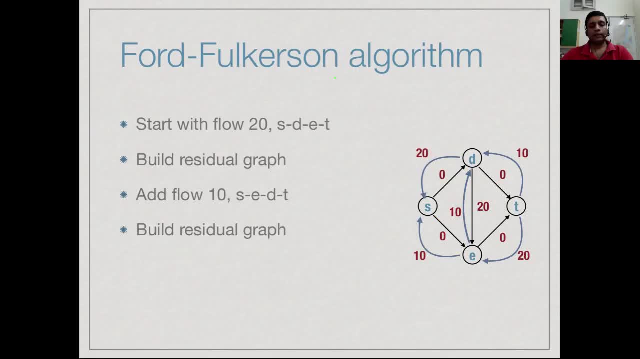 begin with. So I take that 10 and then I build a residual graph. So when I take that 10, these quantities here Which are associated with this edge, gets restored back by 10.. Because the total flow from d to e was 20 in the first round minus 10 in the second round is 10.. Therefore the 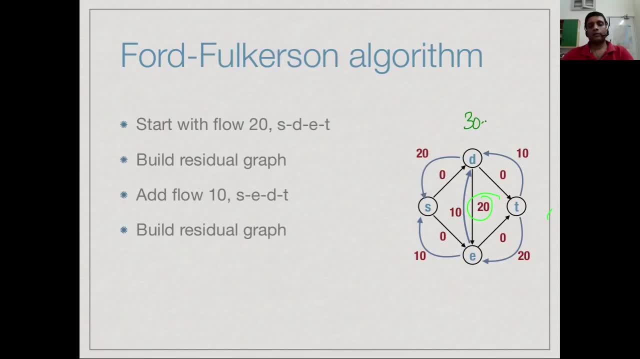 residue is 30 minus 10, equal to 20.. And everywhere else now I have got 0 because I have saturated. Now, if I look at s, there is no outgoing flow possible in this residual graph. So then I say that there are no more feasible paths and I stop. 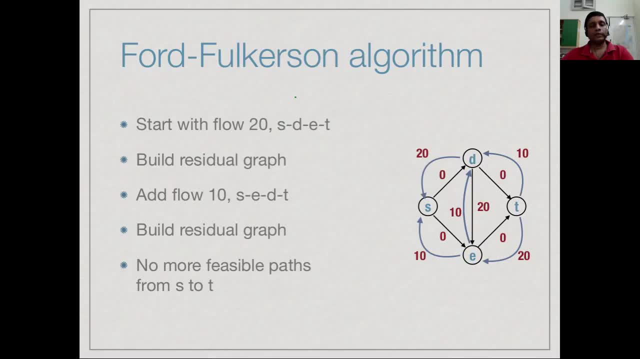 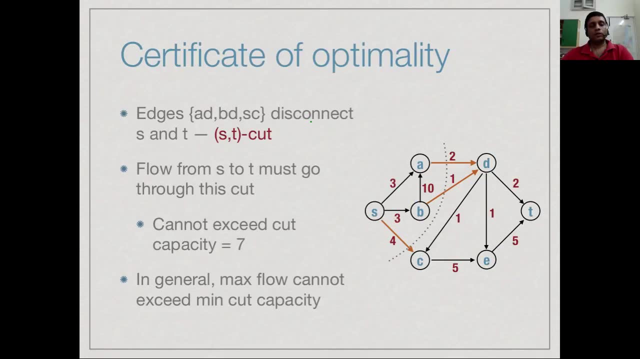 and the residual edges, or if I have been keeping track of the flows, will tell me that I have achieved a flow of 30 in this graph. So, again, if we want to ask a question as to why a given flow is optimal, we can ask for some quantity which is certificate of optimality. So if we 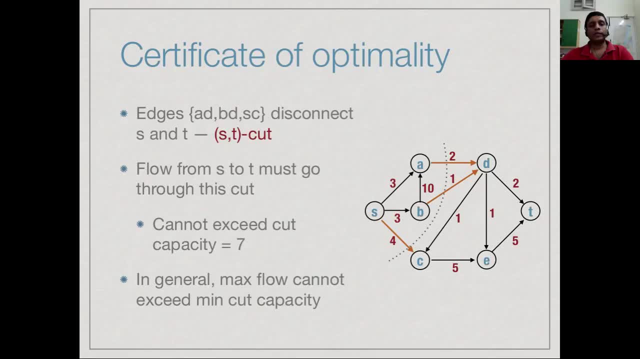 go back to our original oil shipping thing. we claim that we could set up a flow of 7.. So by hand we constructed a flow of 7.. Now let us look at these three edges: the edge A to D, the edge B to D and the edge S to C. If we disconnect this graph by cutting, 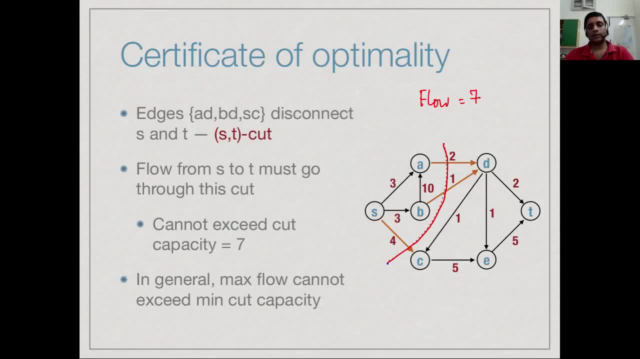 these edges. rather, if we cut these edges, we disconnect this graph. ok, So these three edges form what is called a cut between S and T. Now, in this cut, the total capacity is 4 plus 1 plus 2, 7.. Now, if there is any flow at all, however it flows, it must cross. 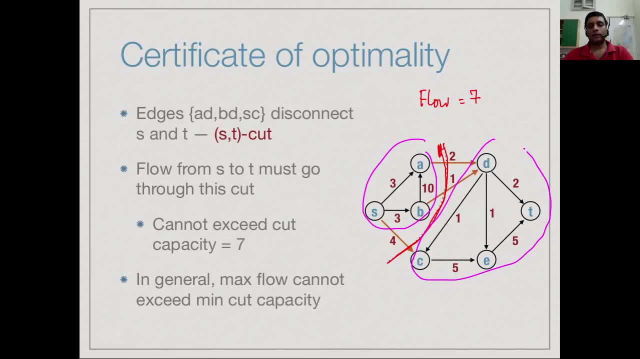 from this side to this side, right from the left to the right. So it can only flow from the left to the right through the edges with that part of the cut, but the cut can only support a flow of 7.. So therefore, our optimum flow can definitely not exceed 7 in this example. 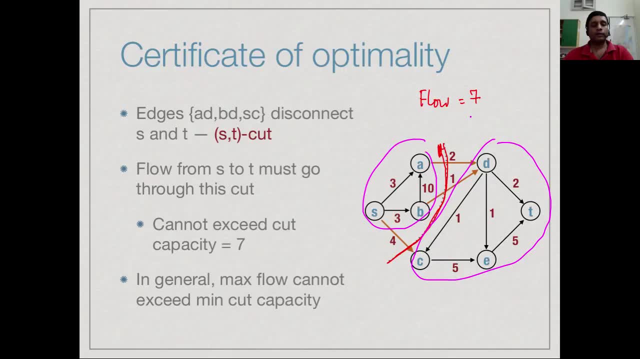 which we have already achieved right. So we know that we can do a flow of 7, but no more than 7 is possible, because this cut will prevent anything more than 7 from flowing from the left to the right. So actually, in this case, this shows us that 7 is optimal. 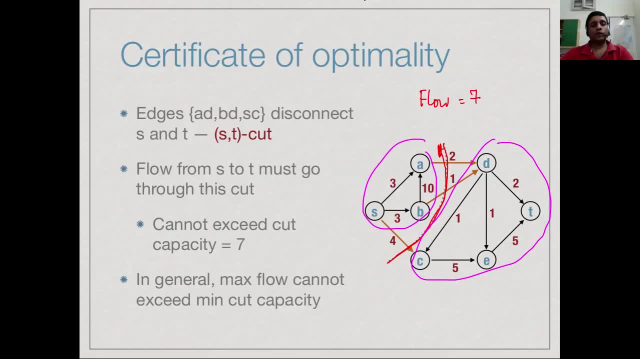 ok, So in general you can look at various such cuts. So a cut is any set of edges which disconnects S from T and you can calculate the minimum cut across all of these right, And it is pretty clear that the maximum flow cannot exceed the minimum cut because it has 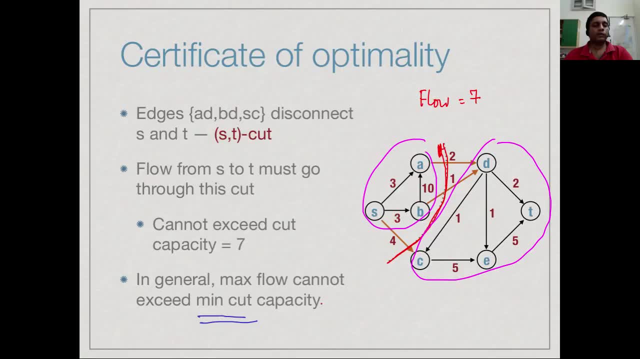 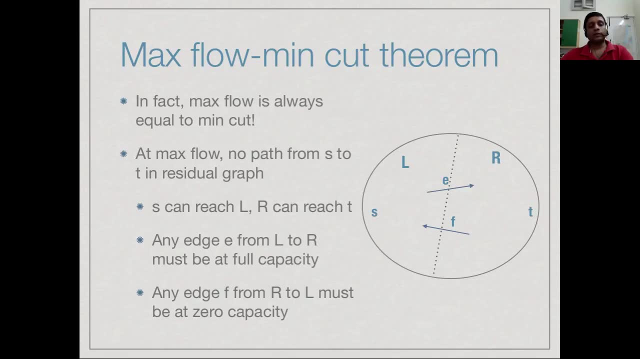 to cross this cut right, So you have to go from one side to the other. it can only take that much capacity, So the flow cannot exceed that. So what is surprising is actually that it will always in this, in this example of that. 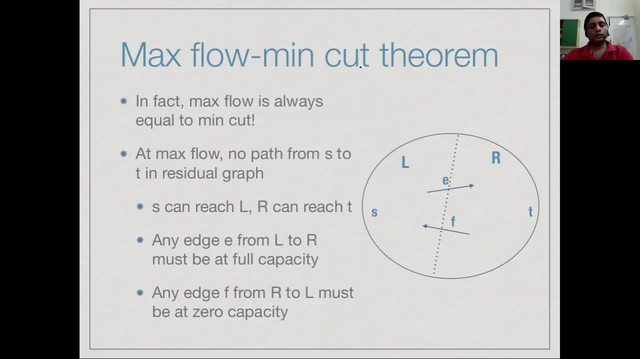 we did. it was equal, but it is always going to be equal. ok, So the max flow min cut theorem says that the max flow is actually always equal to the minimum cut. So here is one way to understand this. So if you look at our LP solution, right? 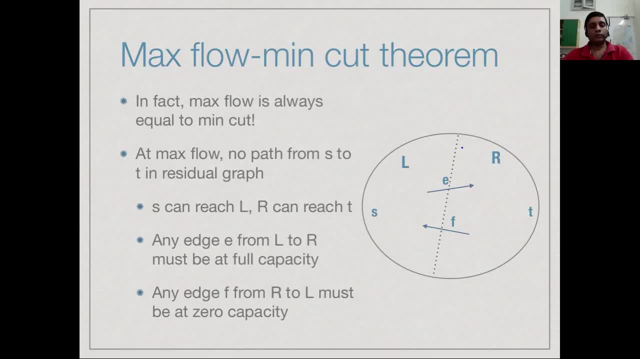 when we achieve the maximum flow, then S is going to be disconnected from T. There is no further path. if I look at edge weight 0 and I remove those edges, then there is no further path, right? So S is disconnected from T. So there is a cut. There are some. 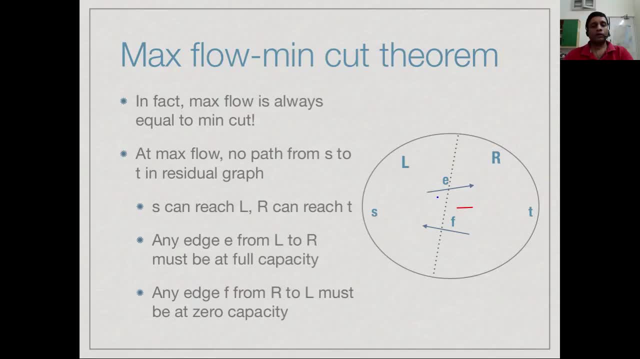 edges which disconnect edge s from t. Now let us look at any edge in the residual graph at that point which goes from the left hand side to the right hand side. ok, So left is everything. So everywhere inside this I do have paths with nonzero weights, ok, and 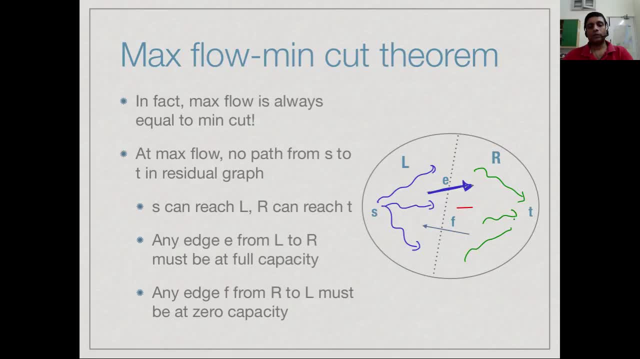 everywhere inside this. I do have paths to t with nonzero weights, So now, but I cannot get from the blue side to the green side. So that means that in the forward direction all the edges must have saturated the capacity right, So every edge from l to r is actually. 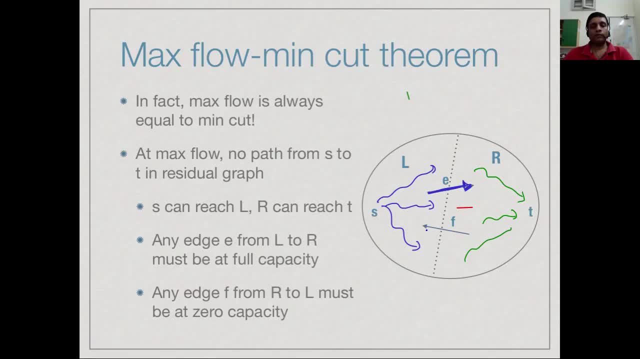 a full capacity. What about an edge? in my residual graph from f to r to l? The claim is that if there was some capacity here, then there would be a reverse edge which goes this way: right, which would be at nonzero capacity. So there would be. 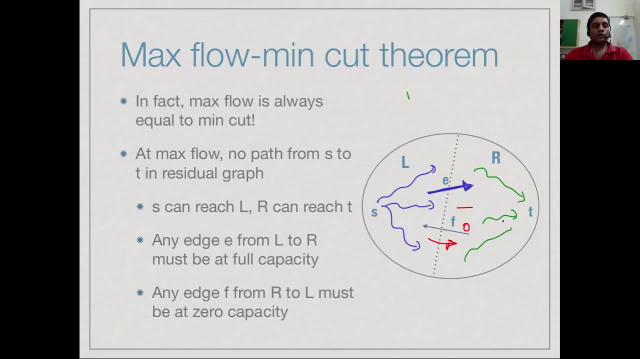 a path from s to t, but there are no paths, So this must be at 0.. So all the reverse edges must be at 0, all the forward edges must be at full capacity. So this gives a not very precise. 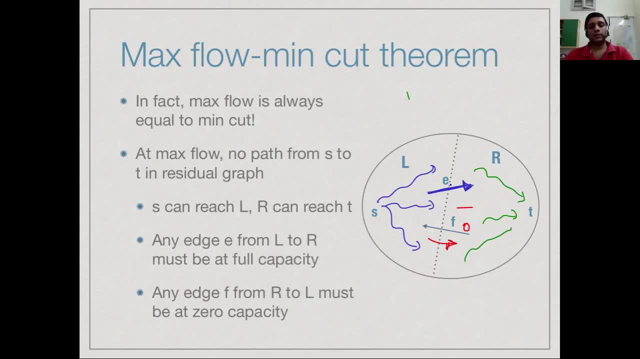 But a reason why the max flow will actually saturate this cut. but this could be any cut, right? So therefore the minimum cut in particular will be saturated and therefore the max flow cannot exceed the minimum cut anyway, right? So the max flow must achieve the minimum. 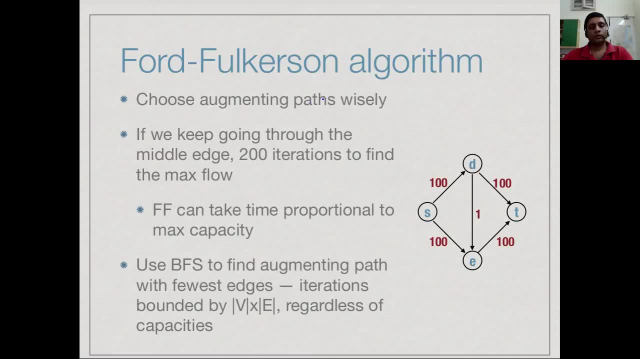 cut value. So one thing that one has to be careful about in the Ford Fulkerson algorithm is the choice of how to increase the path. So remember that in our pathological examples we, instead of going around the diamond, we go through the centre. 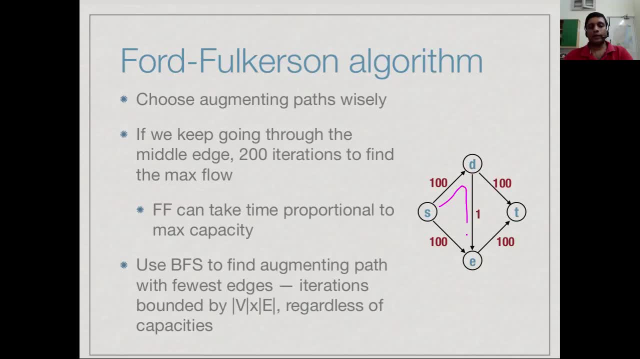 So supposing we keep doing that, then what will happen is that here, after 1 iteration, we will go through the centre and then we will reduce this to 99, this to 0, this to 99 and we will setup a reverse edge of size 1.. Then in the next iteration we will go in 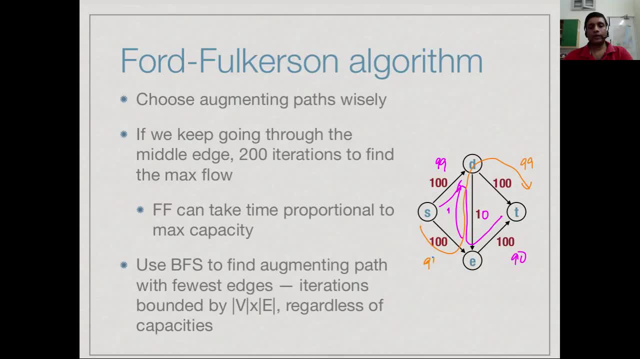 the reverse direction and we will again reduce this to 99, this to 99, and then we will setup this, reset this right back to 1.. So this way we can keep zig zagging. So I will go from 99 to 98 and then down, I will go from 99 to 98.. So it will take. 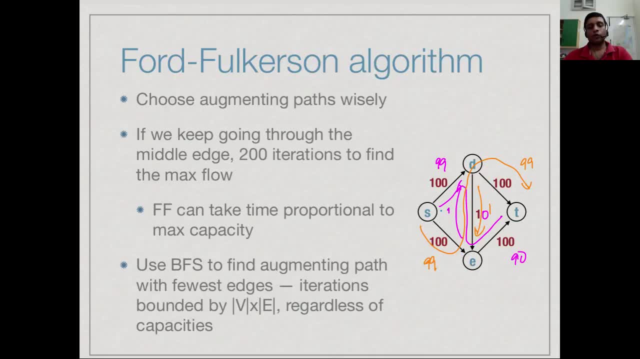 me 200 iterations find this path, that this flow has 200.. On the other hand, it is pretty clear that I could have done it in two iterations if I had been cleverer, because I could have just said initially: there is a path of 200 there and that saturates those two edges and there 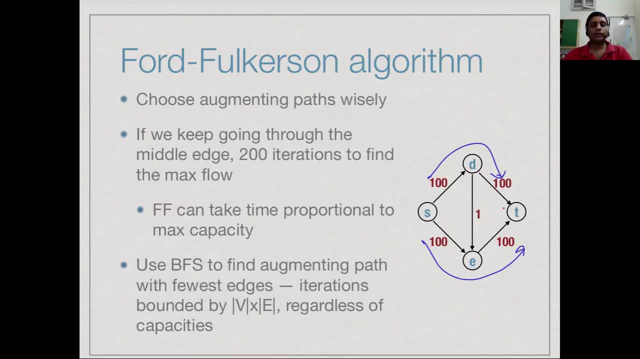 is another path of 100 there and a path of 100 here, So in two iterations I can achieve 200.. So it depends quite crucially on how I pick the path to augment. How do I take the feasible paths which still exist in the residual graph and choose which one to add? 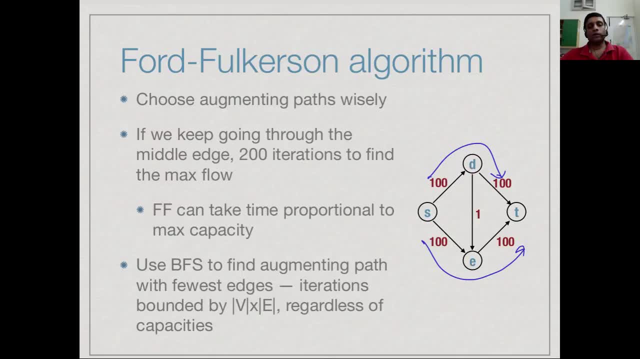 to. So in general, we cannot say anything good and Ford Fulkerson is going to take time which is proportional to the capacity of the edges, which is not a great idea because, although the edges may be large, you might be able to directly say: oh, this edge can take 100, the 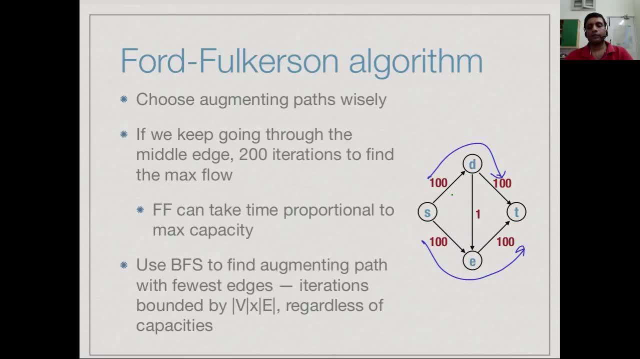 next edge can take 100. So in one shot I can say the whole path can take 100, but if I have to do one at a time then it becomes an extra parameter, not the actual size of the graph, But how do we do this feasible path business.